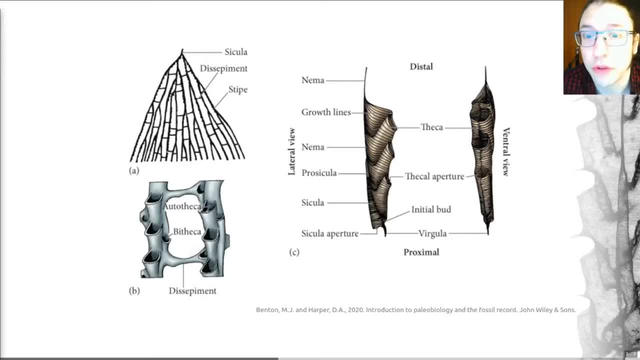 So the structure we see as fossil Graptolites is used to house zooids. It's a thing called the tuberium, So this is the housing of the colony and that was probably collagenous, so made of collagen, like many of our connective tissues within the vertebrates. 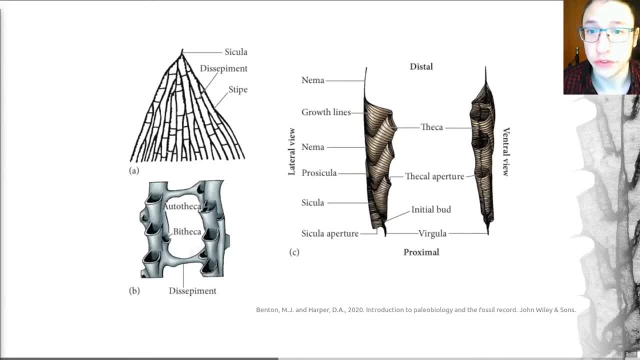 Although Graptolites are abundant and important fossils in many early Paleozoic assemblages, it is notoriously difficult to discover what they're actually made of, And that's because most assemblages occur in black shales that have been either compacted or diagenized. 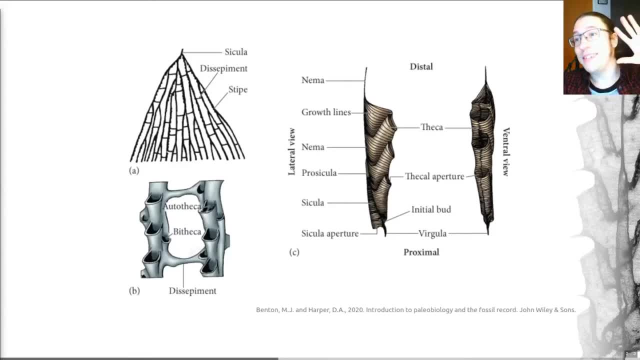 So that limits what we can say about what they're made of. but if we look in detail at this tuberium, this colony housing, we can see, for example, that they have a growth pattern. It's made of half rings that meet in zigzag structures. 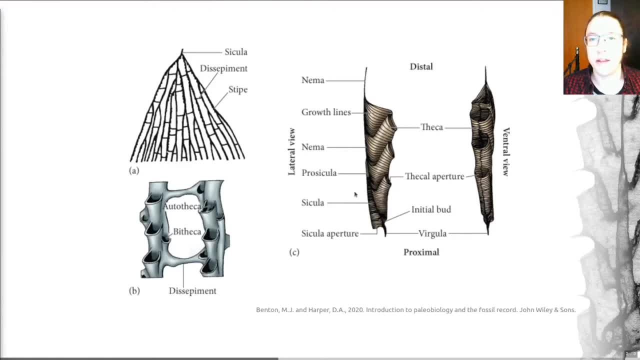 It's most clearly visible in this diagram on the right, Each tuberium represents just one colony, which grew from a small cone called the cicula. So the cicula can be at the top, as in this orientation here, or it can be at the bottom of the organism, depending on which particular group you're looking at. 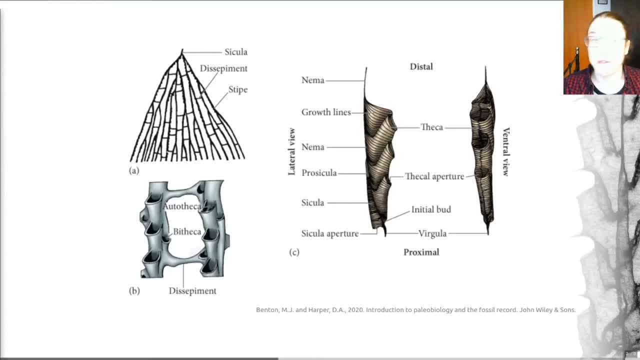 The colony comprises a series of branches- That's true of of all Graptolite colonies, though that number of branches can be one- And these branches are called the stipes. These stipes may be isolated. They may, for example, dangle freely. 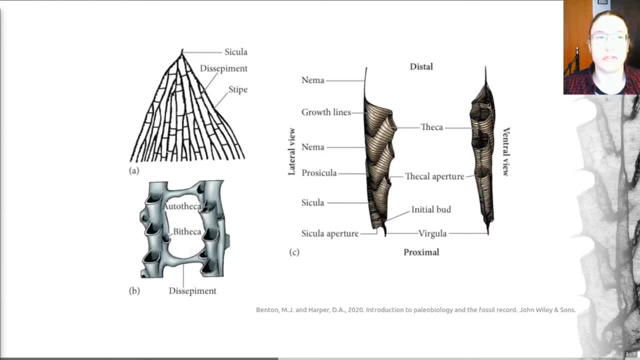 Or they can be linked together by lateral struts, as shown in this example on the top left here, And these are called dissepaments, So similar to the name that you have for cross bits in corals, although not necessarily homologous with those. 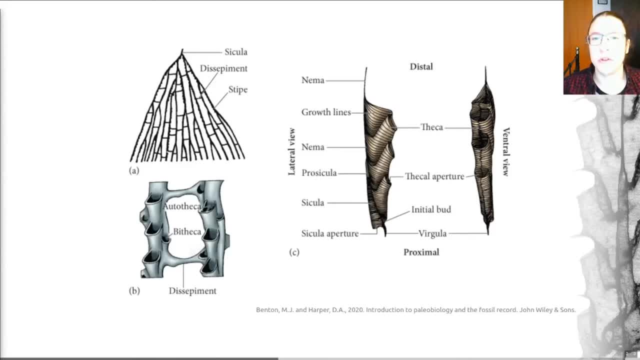 Same word. If you look at the stipes in detail, what you see is a series of roughly cylindrical tubes in which our zooids lived. These are called thecae, So you can see examples both here on the left and here on the right. 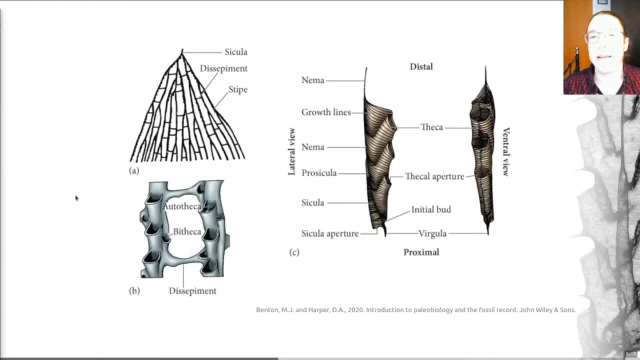 So this one's nicely labeled thecae for you. So thecae is the plural of thecae, So these thecae housed our individual zooids, our individual animals that make up the colony. And just FYI, these animals were genetically identical. 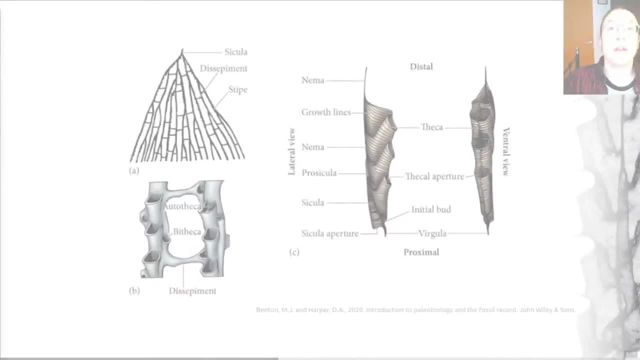 So they are all genetically the same. There are two important divisions that we need to know about within the Graptolites. These are the dendroids and the graptoloids, or dendroidia or graptoloidia. So this does mean that occasionally we have dendroid Graptolites and graptoloid Graptolites. 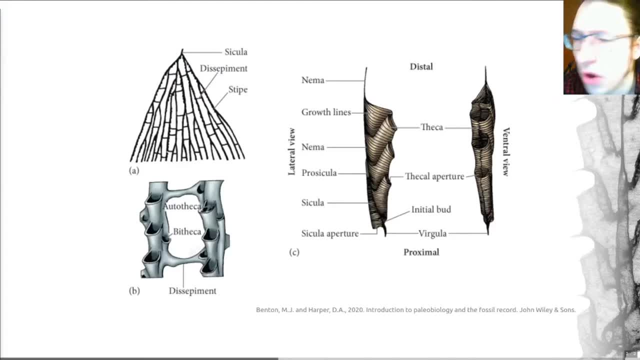 Bit of a mouthful. But just bear in mind that this is just a subdivision of the Graptolites as a whole. The origins and the evolution of this group, or both these groups, are matters of current research. So the dendroidia is the older of these two main groupings. 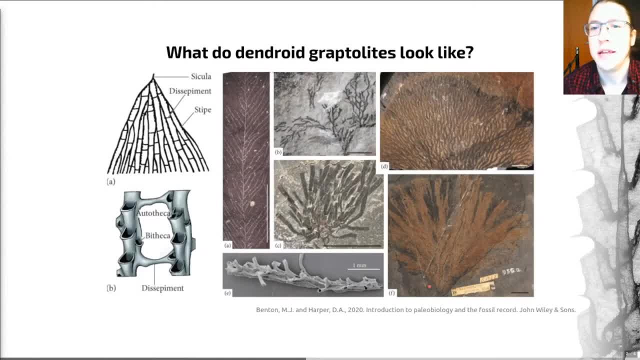 So these creatures appeared in the middle Cambrian and disappeared in the late Carboniferous. They are marked by having a tuberium. So this, this colony structure as a whole that was multi branched. It looks a bit like a bush, even though it's not related to plants. 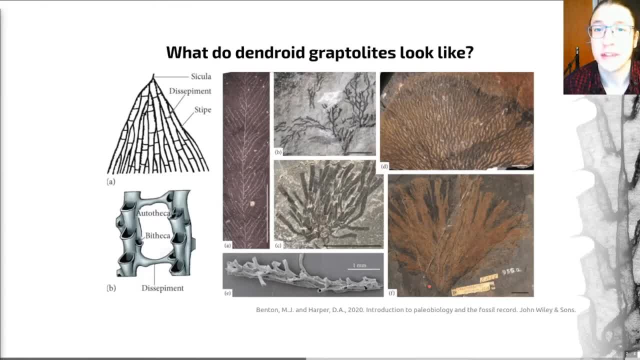 With its many types connected laterally by dissepaments, So that phrase that we met earlier in this video. These creatures have two types of theca of different sizes, called the autotheca and the biotheca. Those names aren't important, but just the fact that there are two types of theca within the dendroidia is useful to know. 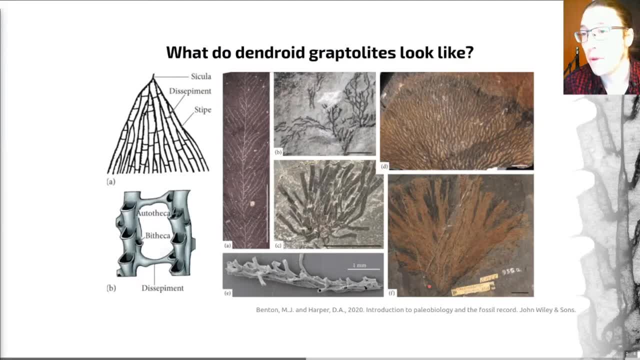 The group as a whole started as benthic- and indeed the majority of the members of this group are benthic- Attached to the seafloor by a short stalk with a basal disc, So that's an attachment disc. In the latest Cambrian, a few genera detached themselves from the seafloor and evolved into a planktonic or floating mode of life. 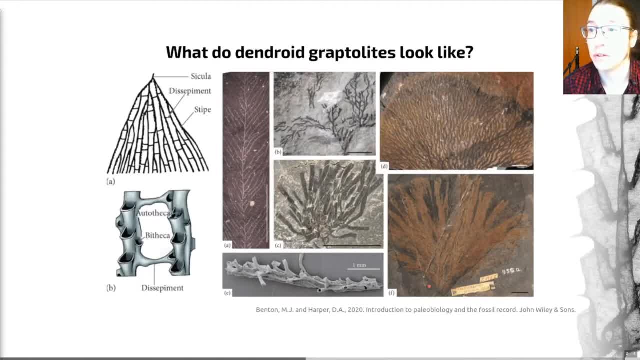 And so that's probably the origin of our Reptiloid Graptolites. The example of our dendroidia are shown on the right here, And these show something. This shows some of the range of form within this group. Bear in mind that all are kind of erect growing forms attached to the seafloor, apart from C. 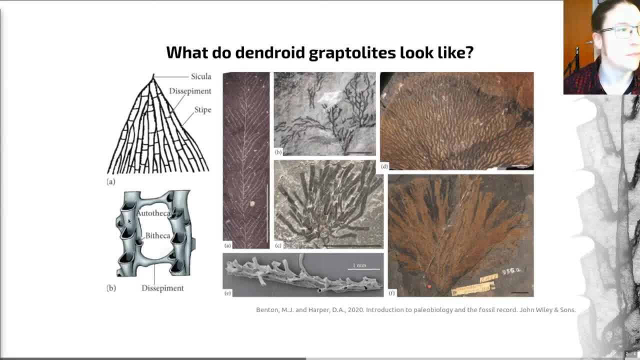 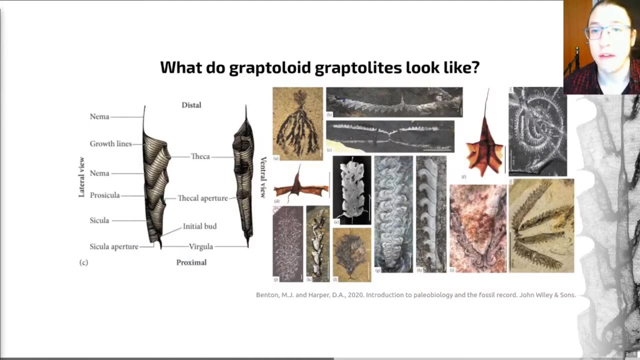 This creature in the middle here. that was an encrusting form, But these two on the right are the kind of structures that I associate with my typical member of the dendroidia. If we move on to our other group, the Graptoloid Tuberium, 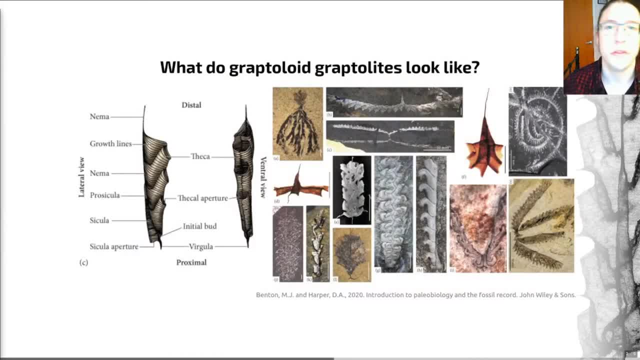 So this is our Graptoloid Graptolite. It appears simpler than the dendroid Tuberium. It comprises an initial cicula that's divided into different areas, But essentially that leads to a spine at its apex, which is often a long, thin structure and is called the Nema. 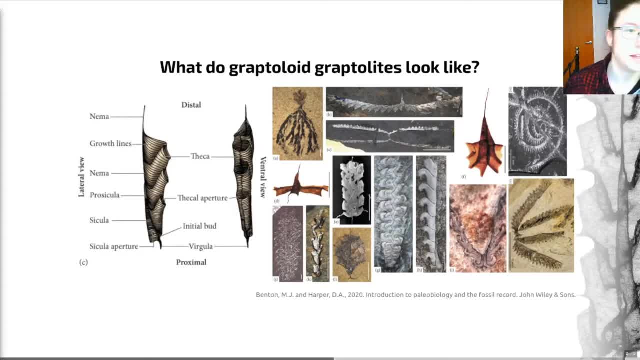 So you can see it labeled here. Our cicula is down here on this creature and this structure goes all the way up the back of this colony. I say back. that's not an anatomical description, just the left hand side of this drawing. 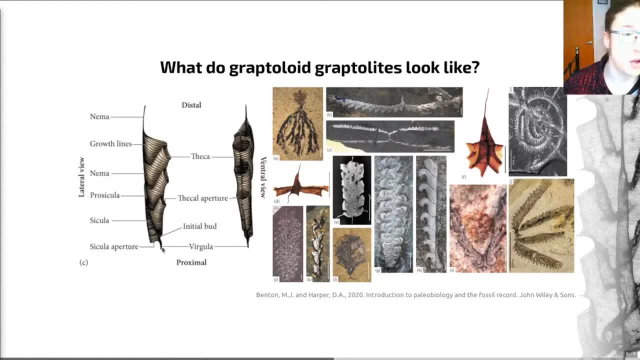 This structure, the Vigella, projects below the cicula aperture and is only present in some species. It's not particularly important. The thecae grew out from the cicula and subsequent thecae grew in sequence as the Tuberium developed, So you've got thecae being added as this thing grows. 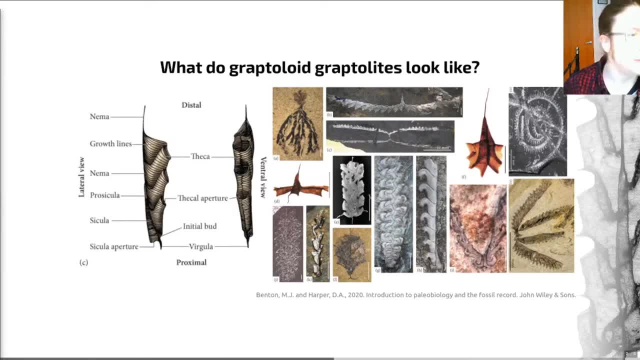 There are a wide range of forms in this group, As you can see from these images on the right hand side here, The taxonomy within the Graptoloids is based on the number of stypes, those branches of the colony as a whole. 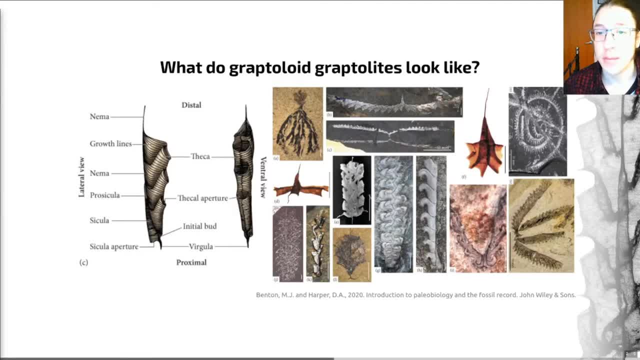 their mutual attitudes and the shape of the thecae on them. So those are three things that are really useful in taking this really diverse group of creatures and adding some sensible organizations to them. So only some of this disparity is shown on the right hand side. 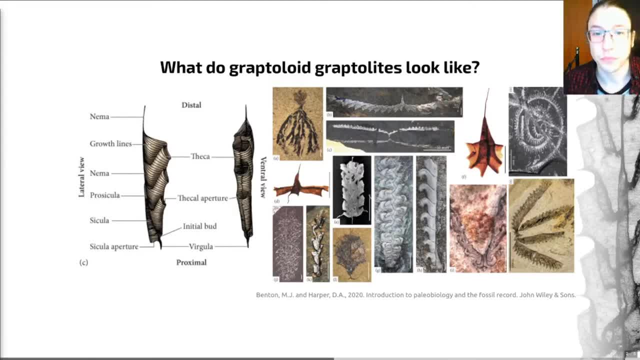 So only some of the range of variation within the group. But you can see, even within this limited collection you've got everything from more than two through two to one type within these colonies, And some of them even look coiled up. This actually makes a bit more sense when we put it into some evolutionary context. 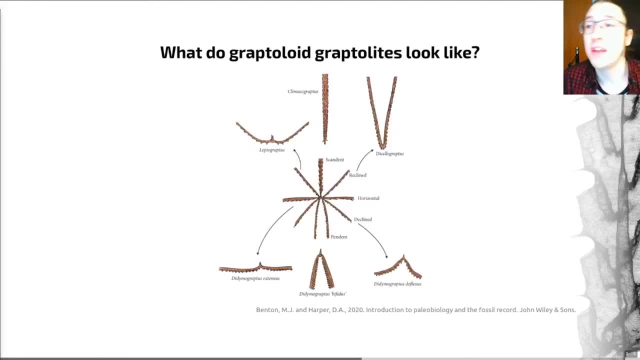 But in order to put these into that evolution context, we just need a tiny bit more terminology. So in Graptoloids, in fact in one particular suborder, the Dicograptids or Dicograptids, the stypes can take a number of different positions. 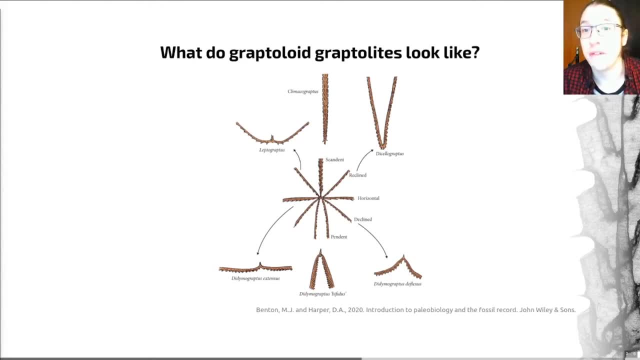 All of which, of course, because this is paleontology- have their own name. So this group actually underwent a radiation in the Ordovician And we have this variety of symmetric Graptolites with between eight and two stypes that appeared. 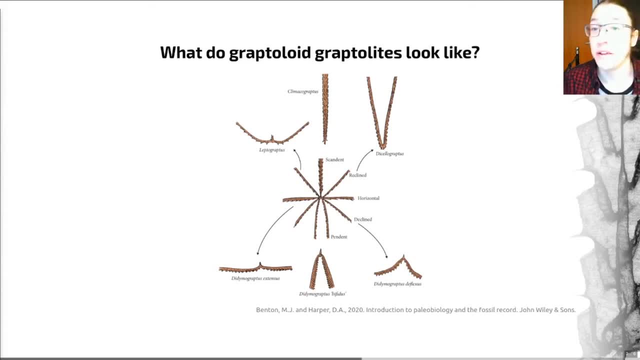 in relatively short succession after each other. We can define their attitude, ie how the stypes are related to each other in space, as pendent, so hanging downwards, Declined, so actually starting to separate a tiny bit, As horizontal. that's exactly what it says on the tin. 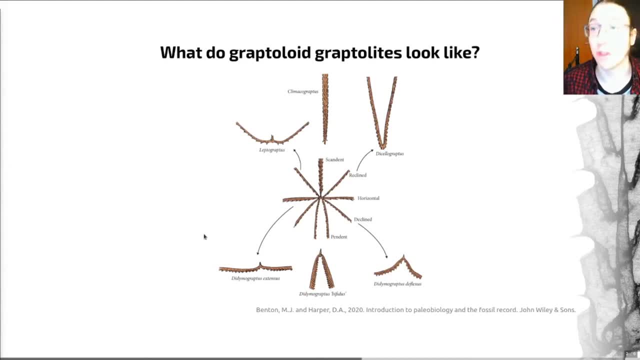 There's an example of a horizontal species here, As reclined. this is the point at which the stypes have gone past the horizontal and have started moving upwards, Or scandent, where they actually meet back to back, as it were, And we start getting a single structure hanging downwards. 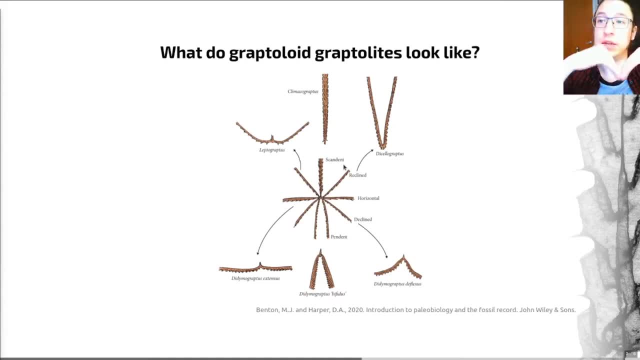 So all of those different attitudes of the stypes exist in different species. This diagram shows examples of those arrangements with example species of each. But as a general point, with this diagram what we're looking at is the evolution of the group roughly. There are obviously exceptions. 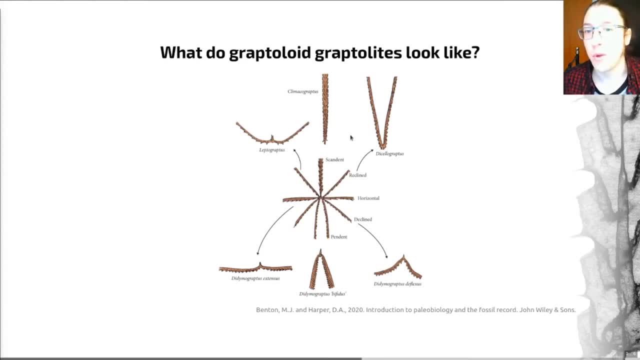 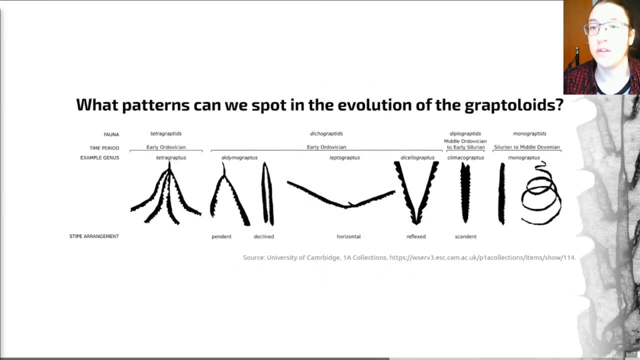 But as we travel from the bottom to the top at the top of the diagram, we're also travelling through the Ordovician in time, And that's because there's a really famous and well-studied evolutionary change within this group throughout the Ordovician that is associated with this radiation. 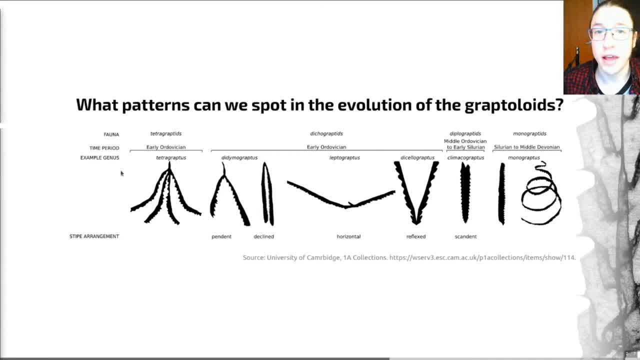 So Tetragraptus- and this example on the far left here of this image that I have sourced from the University of Cambridge- was common in the late-early Ordovician, And it typically had four stypes arranged Either in horizontal pendent or reclined attitudes. 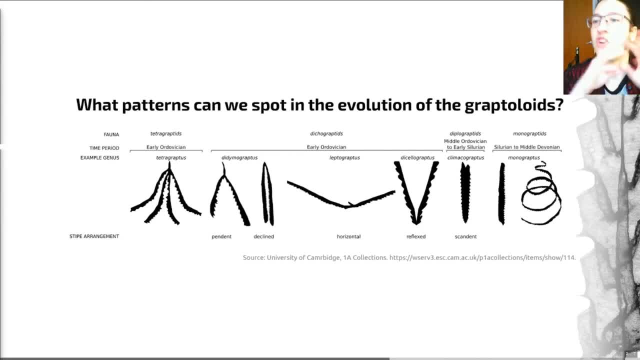 It had simple overlapping thecae, So we're looking at a kind of dangling form that's relatively simple Around. this time we get a genus called Didymograptus appearing, So this is marked by a twin-styped, or otherwise known as biramous form. 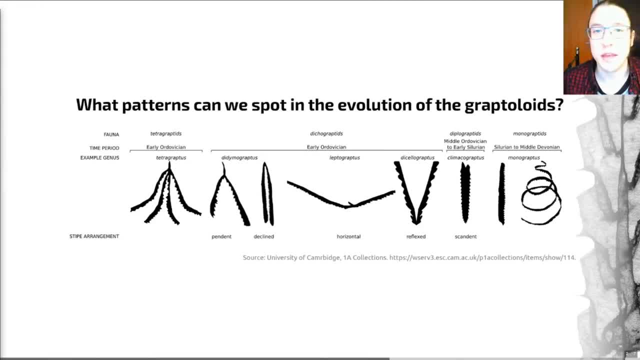 so only two stypes rather than more, which appeared shortly afterwards. These types could be horizontal pendent or reclined in their orientation, And again they had fairly simple thecae. But then we start seeing as we move through the Ordovician. 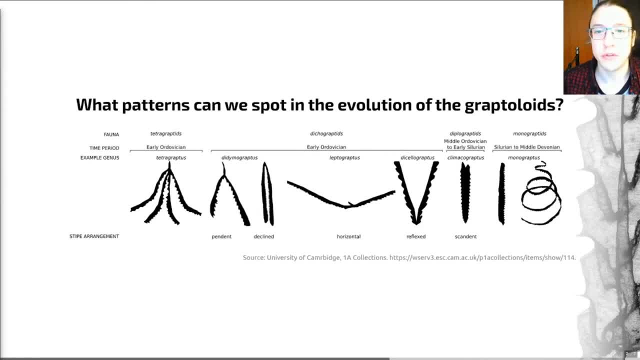 tags that are more horizontal in the arrangement of their stripes. So this example is Leptograptus. here in the middle We then have examples that start appearing like Dicellograptus, which has a pair of stripes that adopted a reclined 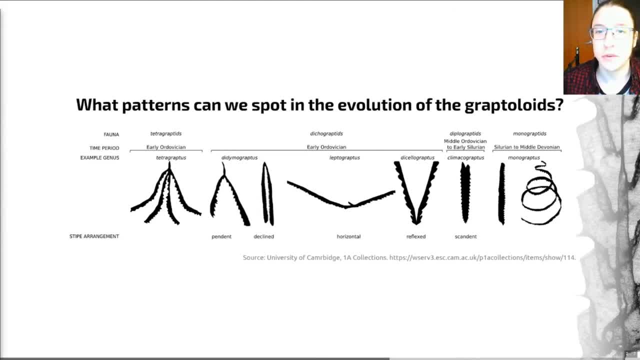 or sometimes called reflexed, as here, attitudes. Often the branches of these individuals were curved or even coiled. A thecae were characterized by more complex form than these simple forms I talked about earlier. They had, for example, extravagant sigmoidal shapes and incurved apertures. 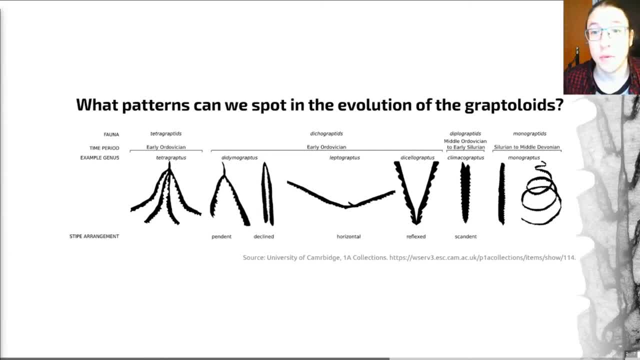 so the openings were very, very complex. By the middle Ordovician and through to the Silurian, we start seeing scandent forms where the thecae are on the outside of the cult colony appearing. So these are the examples shown on the right. 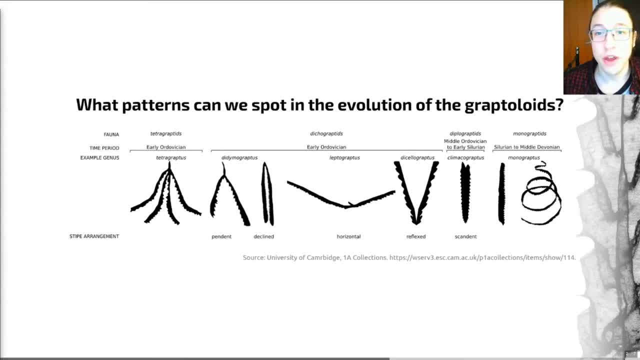 Finally, by the Silurian, we start to see forms where one of those types has been lost. Then you get a thing called a uniserial, scandent form, such as Monograptus shown on the right here. So this one has thecae on both sides. 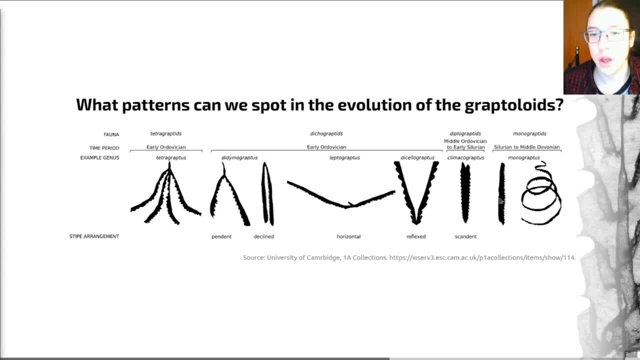 this one's got thecae only on one side. These creatures had either a straight, as seen here, or a curved tuberium and a nema embedded in the dorsal wall that projected distally. So Monograptids. these creatures on the right-hand side here. 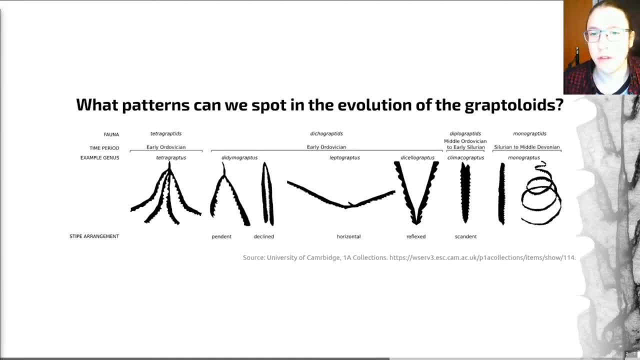 dominated Silurian Graptolite faunas And despite their, I guess, apparent simplicity, this group evolved a huge variety of forms. They're most easily recognised through their faecal shape and arrangement: The last Graptolites, and indeed Graptoloids. 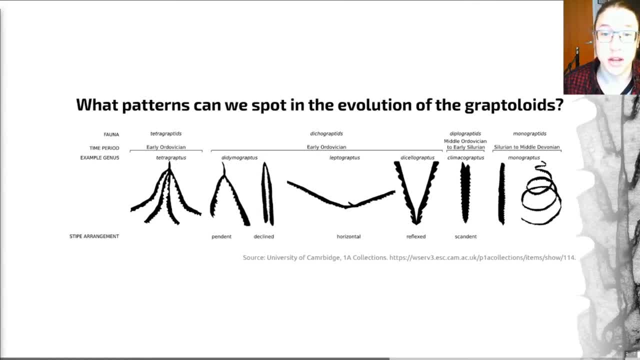 appeared during the early Devonian in China and Eurasia and North America in terms of new species that we see in the fossil record. But remember there are arguments going on that some groups that are still alive today may actually be members of this group. 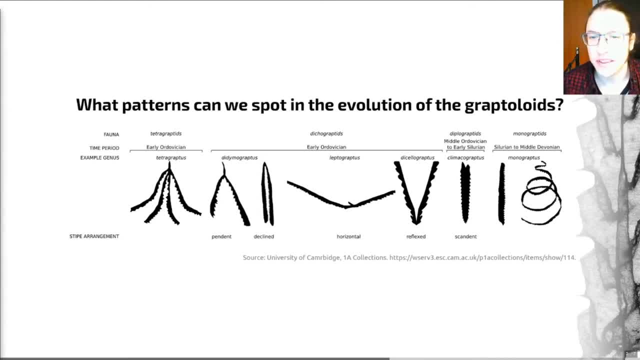 If so, we've got this very long ghost range. This is a really distinctive and quite famous example of evolution in the fossil record that at a glance can often tell you roughly where you are in the Ordovician or the Silurian. 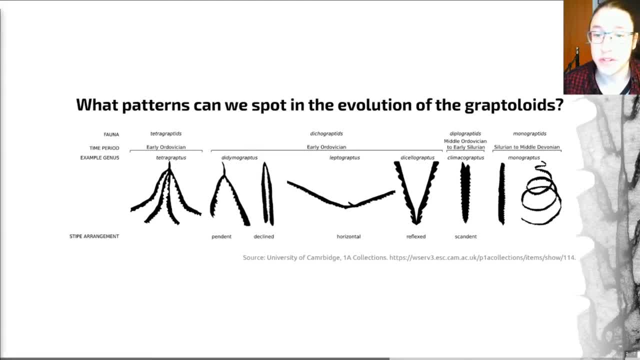 An interesting question which we may want to consider is: why is there this trend towards the reduction in the number of stypes? It could be that the simpler stype configuration was hydrodynamically more stable and better adapted to turbulence. That's one idea that has been published. 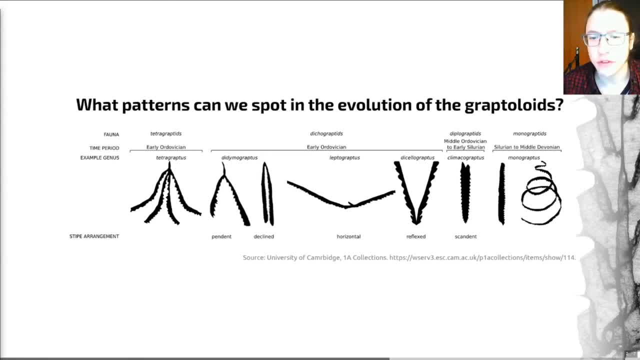 It could be that it aided the motion of the Graptolites through the water column when they were feeding. It could have been to prevent the interference between thecae on adjacent stypes, providing a simpler, more efficient colony structure. Or it could be a combination of any of these three things. 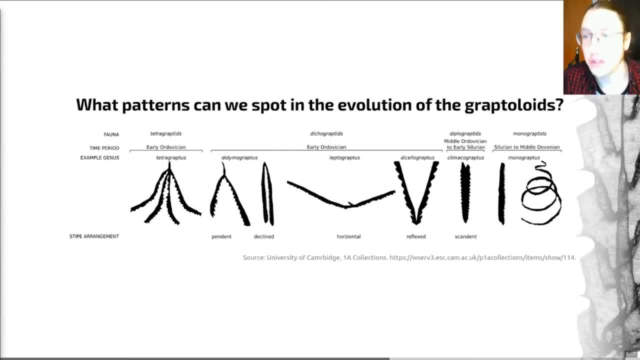 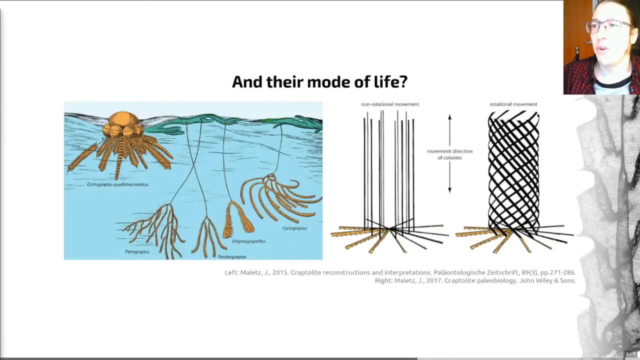 We really don't know at the moment. so that's why this is a really interesting group to learn about, because there are lots of unanswered questions. I think it's safe to say that this is true also of the mode of life of these creatures. 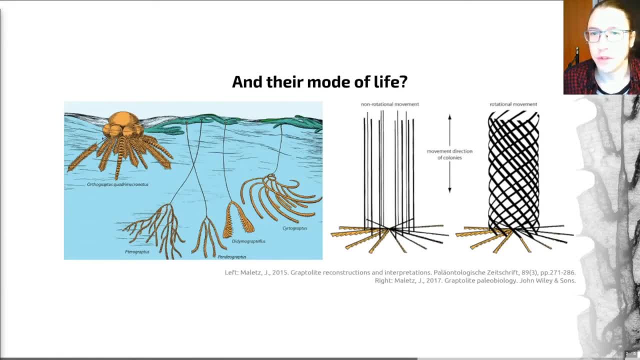 It's far easier with dendroid Graptolites, where they were either benthic- so we know they're attached and they live in the seafloor- or the occasionally planktonic. the mode of life of Graptoloids is more controversial. 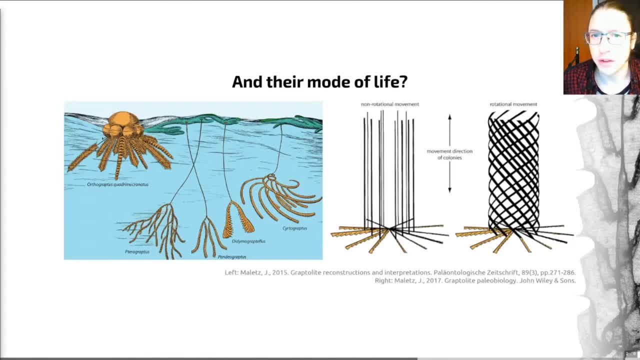 So there have been ideas published in the past that these creatures were attached to rocks or seaweed. This is what's shown on the diagram on the left of this slide. here is also my title slide and is now widely believed to be incorrect. 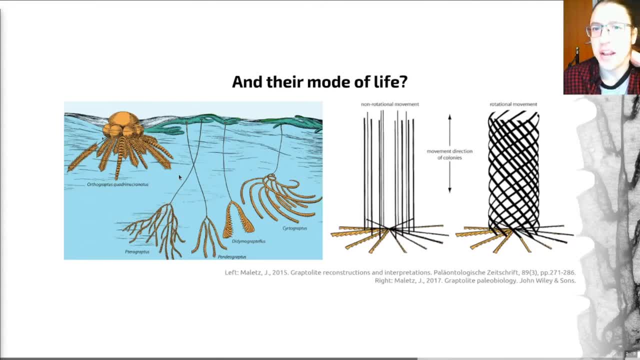 Researchers have rejected this idea because there is no evidence for attachment to rocks As such. we now think that planktonic Graptoloids- so the Graptoloidea- lived unattached in the oceans. We think they were actively moving through the water column. 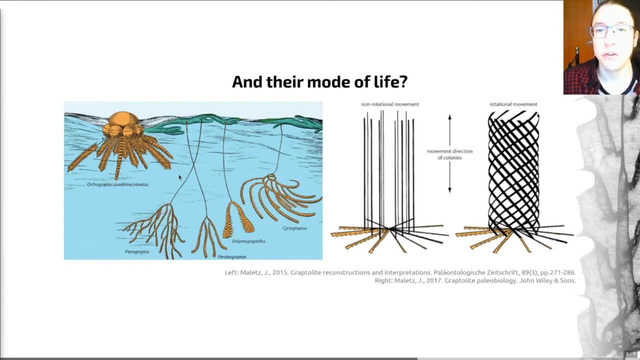 filtering water to gather food. It's now relatively widely accepted that these colonies can move both up and down in the water column as they so wished and it seems likely. they're different from the rest of the world, So the distribution in the water column